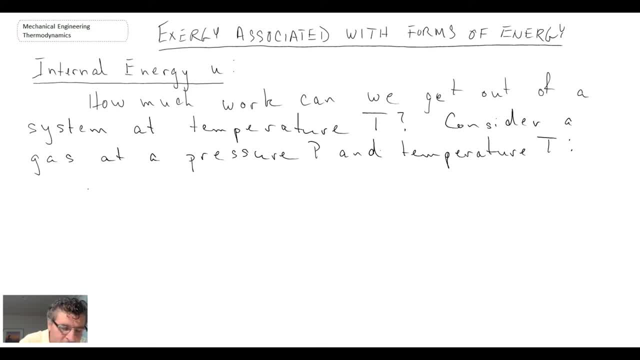 we're going to in order to study this is: we're going to consider a gas and a piston-cylinder device and we're going to assume the atmospheric pressure as p-naught. The gas is inside of our piston-cylinder device and we will assume that it is at 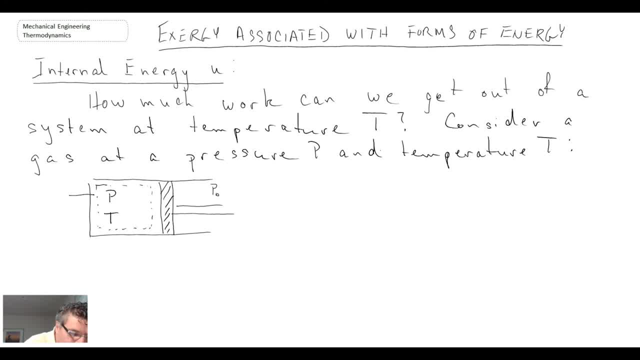 pressure P and T, and we'll call the boundary there 1.. Now what is happening is, if this gas is at a higher temperature, let's assume that a couple of things could take place. One is the gas could expand and, in the process of, 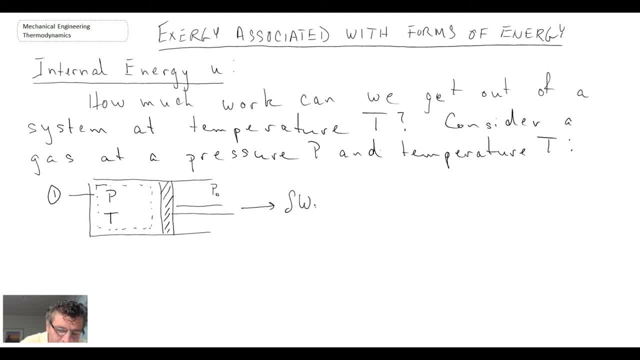 expanding. what we are doing is we're doing boundary work and we'll be interested in the amount of useful boundary work coming out of that. And at the same time, if the gas is at a temperature that is hotter than the surroundings, and we'll say the surroundings are at temperature T-naught. 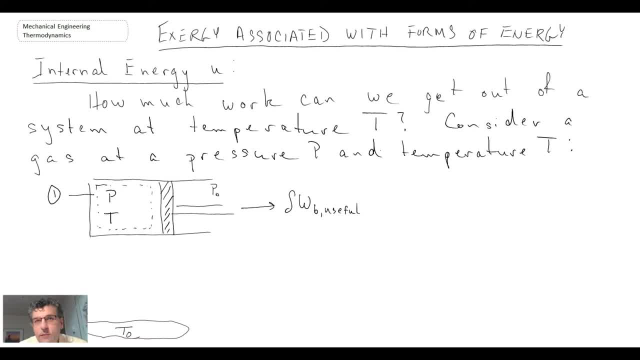 then what we can do is we can put a heat engine between the gas at the hotter temperature and the surroundings. So what I'm going to do is I'm going to sketch a heat engine here and the heat loss rate from our gas which is at a hotter temperature. we will denote that as 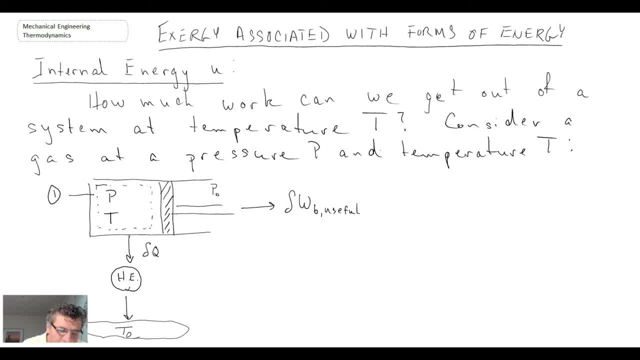 delta Q, Some of the heat will be converted into work and some of it can be rejected by our heat engine, and then what we have is we have an amount of work coming out here with our heat engine. So that is a scenario that we're. 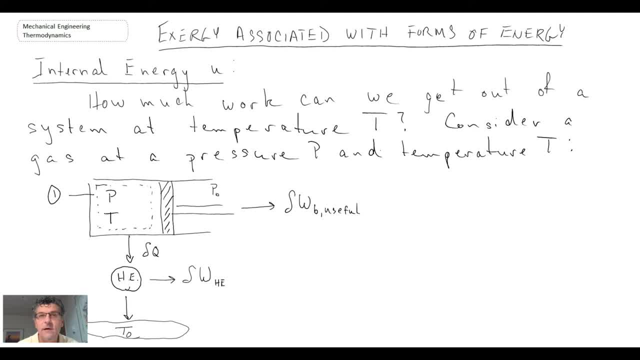 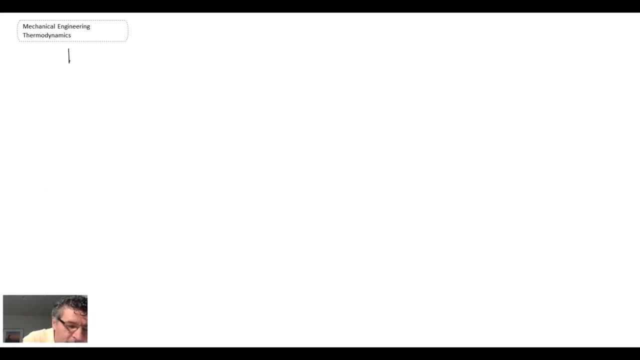 going to examine. What I want to do now is apply a first law analysis to this system. We will then ultimately come up with a form for exergy associated with internal energy. So taking a look at the first law applied to the gas within the 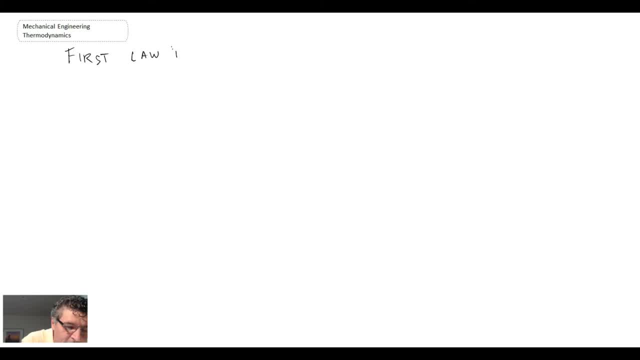 piston cylinder device. I denoted that with boundary 1.. The first law to begin with for a fixed mass system is in reference to heat transfer. Now, what we're going to assume is that the piston cylinder device is not moving, So kinetic energy and potential energy will drop out. 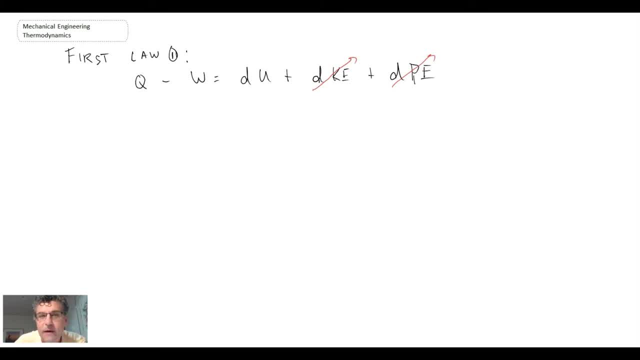 The other thing. remember, in my schematic for the piston cylinder device we had delta Q and delta W. Now the heat was leaving the piston cylinder device and with our convention of heat transfer into a system being positive, that is going to lead to the heat transfer. 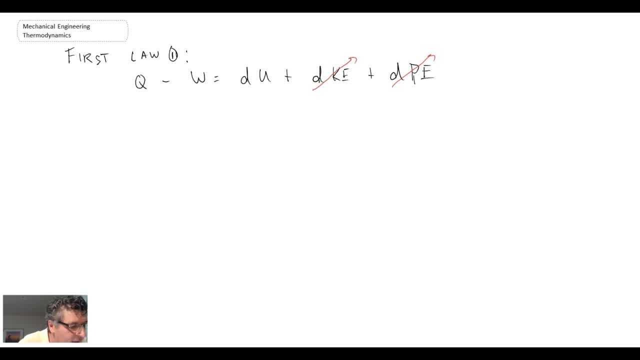 that means that the heat transfer is negative. so I can write minus Delta Q. now it was doing work, so that is positive, so it's minus Delta W is equal to the change in internal energy. now what I'm going to do with the work term. I'm going to expand that into useful work and work being done on the 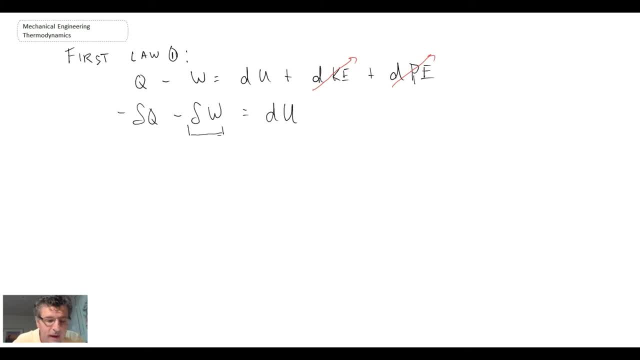 surroundings. remember, when we do extra-g analysis, we need to take into account the amount of work that is being done on the surroundings. so let me expand Delta W so we have useful boundary work and then we also have the work that is being exerted upon the surroundings. and given that it is an 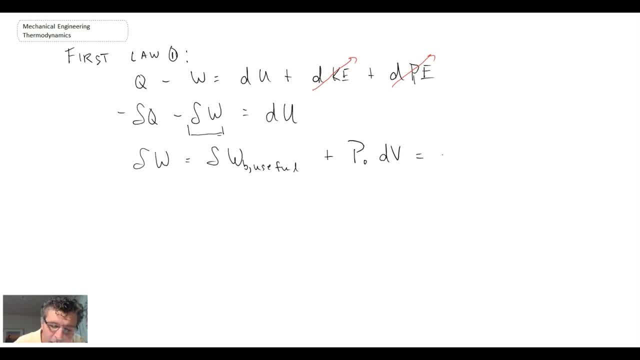 expanding piston cylinder device. the useful work is going to be the pressure above the atmosphere multiplied by the change in volume, plus the work done on the surrounding atmosphere. so the reason why I'm subtracting off the p-naught here is I want pressure above the surrounding atmospheric pressure, or our dead. 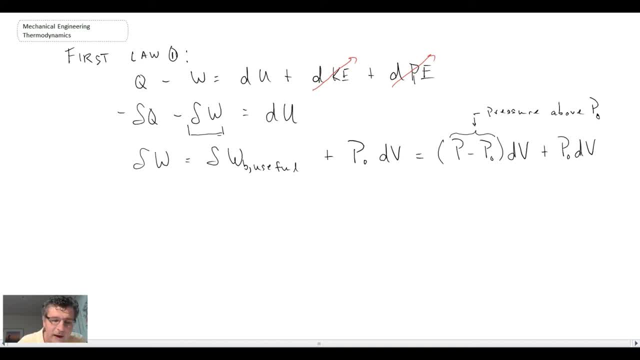 state pressure p-naught. so with that, what we can do is plug this term for the work into the first law, and what we end up with is this equation. so we will label this equation one. that's the first thing that we will consider. the second thing I want to 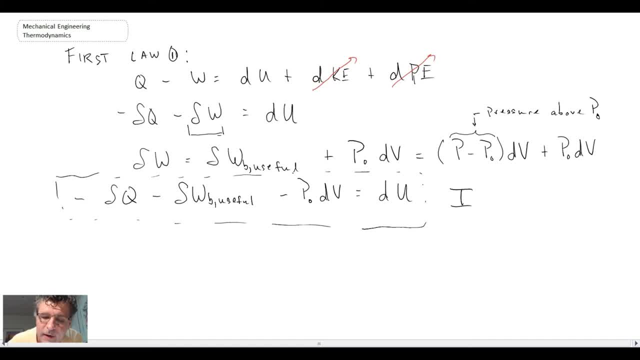 consider is the work going through the heat engine, because, if you recall, with our piston cylinder device we also had a heat engine. so let's take a look at the heat engine and what we're going to do is we're going to try to quantify the work coming out of that heat engine and what we're going to 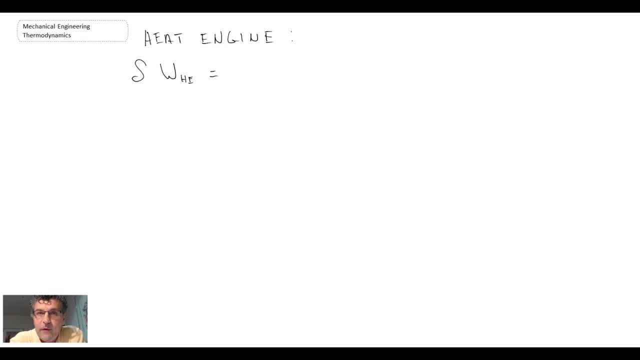 assume is that we have a reversible heat engine, so that would be perhaps the Carnot heat engine or any other heat engine that is reversible. and in order to determine the work coming out, we look at the thermal efficiency for a reversible process, times, the heat transfer coming through that heat engine, which is delta. 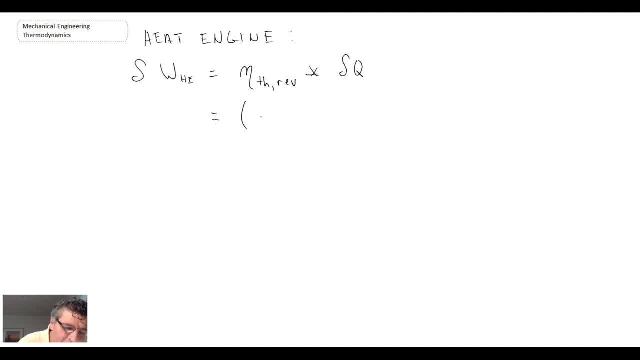 Q. we know that the thermal efficiency for the reversible engine can be expressed in the following manner: where T is the higher temperature of our gas and t-naught is the surrounding temperature, and so what we can do is we can expand this. now. the first term here this is heat flow into the heat engine. 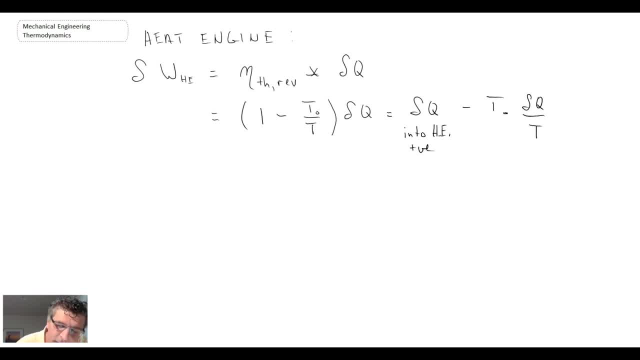 and it is positive. the second term here, the one with the delta Q over T. this heat is crossing our boundary one and consequently it is considered a negative term. so with that, and what I will do is I will introduce the definition of entropy for the delta Q over T, which we saw earlier in the course. 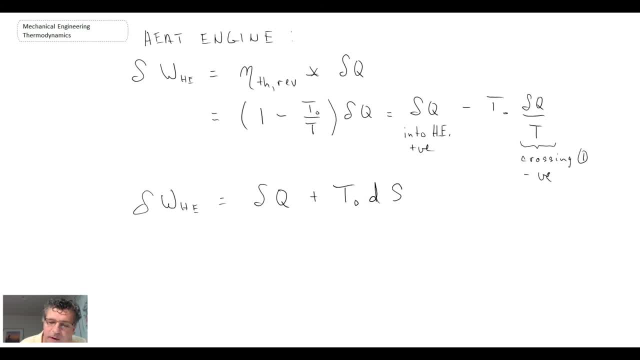 and we obtain that expression. so the trick with that one is the fact that the temperature transfer across one is negative and consequently this term becomes positive, and with that I can now rearrange in terms of delta q, and I will call this equation 2. so what I'm now going to do is I'm going to sub equation 2 into 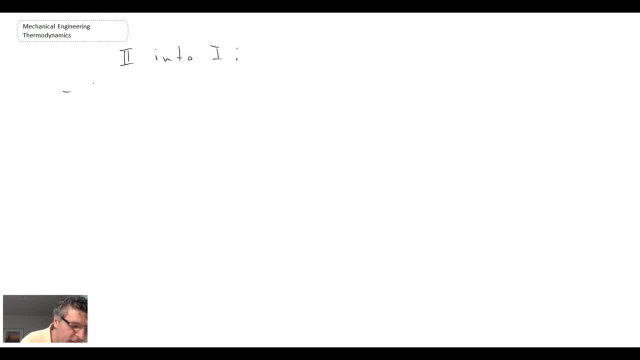 equation 1 and with that we obtain the following expression: today we're going to call this equation 2 c if we just reduce itself for KM and we're facing here through the equation. there we go by removing two versus two-, Squad, one in the end to the 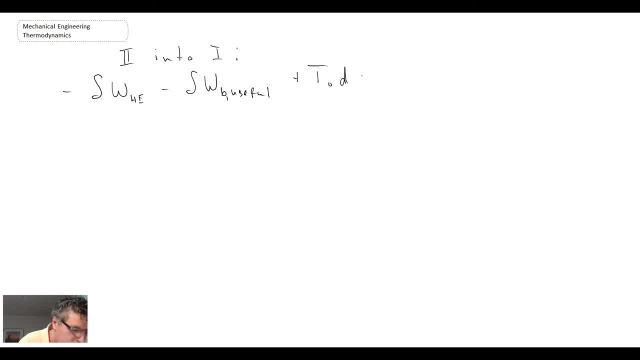 cosine of X: 1. Galawka is going to do a competition here. we are going to leave the ultimate off position of T and then, as we him both go through it again, we are going to do S t to by d over forever spread to the upper quarter. 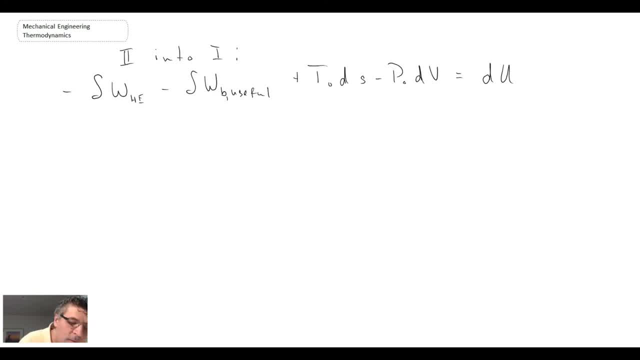 I'm going to change my webinar quite a bit lately with this accountant, but because I decide now all those ng Naturals are going to be fingers, let's complete a Scheduleplan, which is by putting in the Integral value of T, which means that we're going to add certain, which of these are IDs and the names of the. 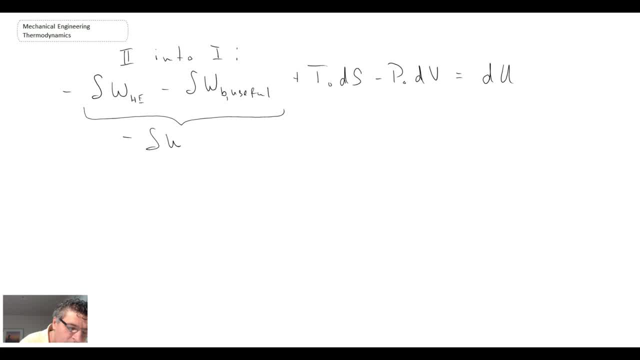 number of numbers that are turned over, which might change this, Oscar, just for example. What I'm going to do is combine the two forms of work, both the heat engine as well as the boundary work useful, into what we will call the total useful work coming out of our gas. 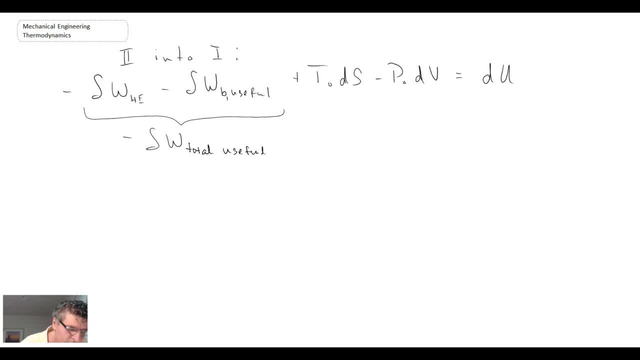 pressure P and temperature T. There we have an expression for the total useful work coming out of our internal energy. what we're going to do is we're going to integrate this with respect to the dead state. So we're integrating from some arbitrary temperature T to the dead state, which 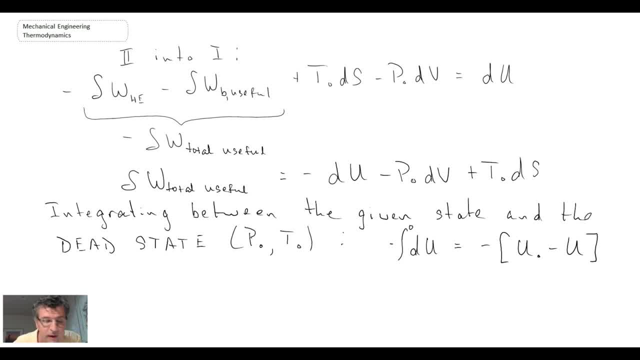 is zero or T naught, and we'll use the subscript zero to denote the dead state. So let's take a look at what happens when we integrate that. We then get the total useful work to be equal to the internal energy change with respect to.